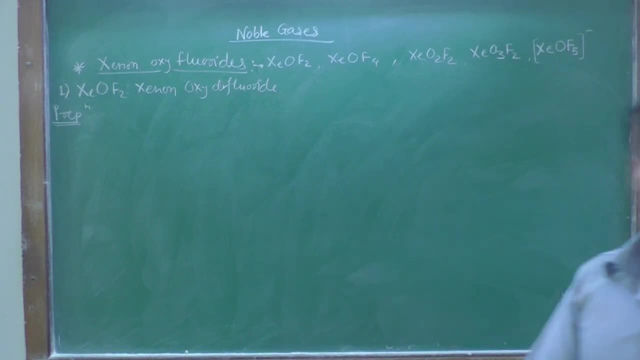 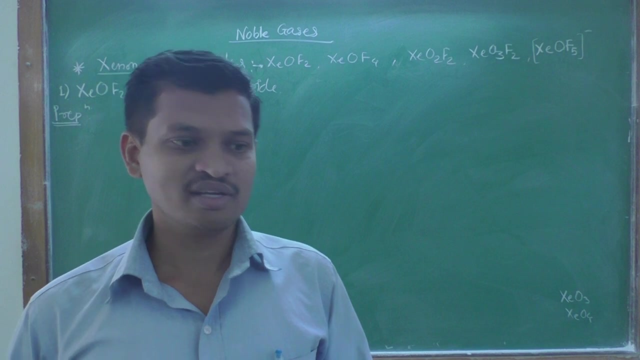 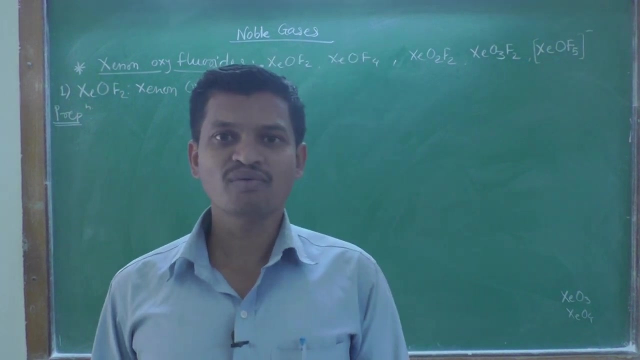 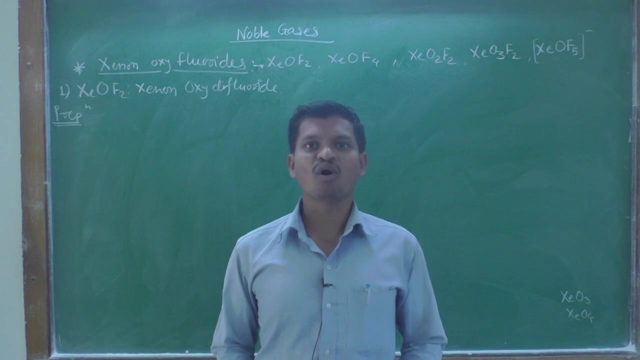 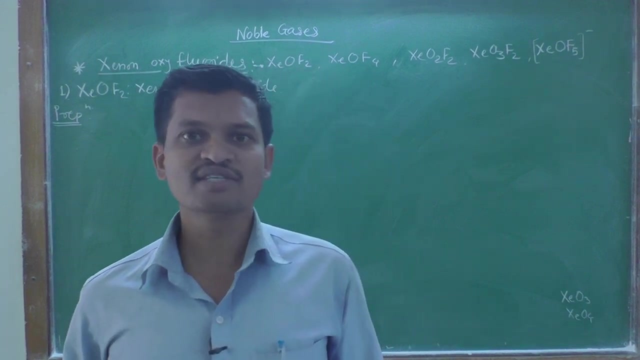 Hello, dear students, very good morning to all of you. Dear students, here we are discussing the chemistry of noble gases and in that we have learned about the compounds of xenon. Xenon is mainly forming three types of compounds. These are xenon fluorides, xenon oxides and xenon oxyfluorides Means when xenon is combining with the oxygen and fluorine in different proportions. it is forming xenon oxides, fluorides and oxyfluorides. Today, let us start. let us discuss about the xenon oxyfluorides. Xenon, combining with oxygen and fluorine, mainly forms three to four types of compounds, and these are xenon oxydifluoride, xenon oxytetrafluoride, xenon dioxydifluoride, then xenon trioxydifluoride and xenon oxytetrafluoride. 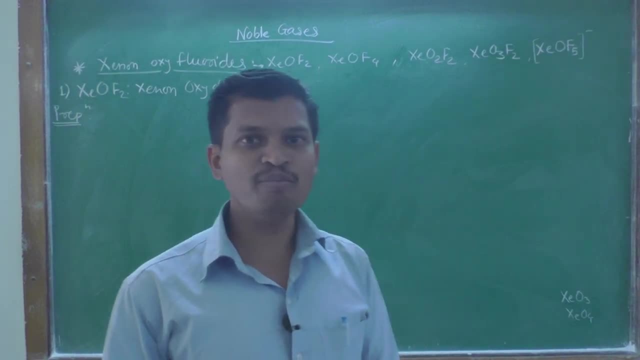 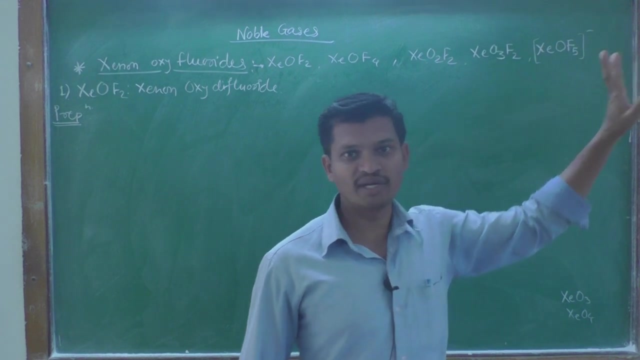 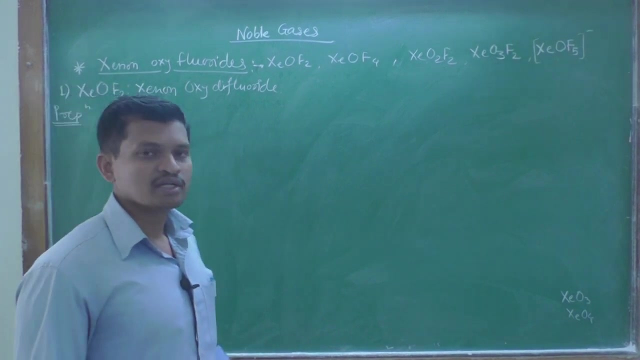 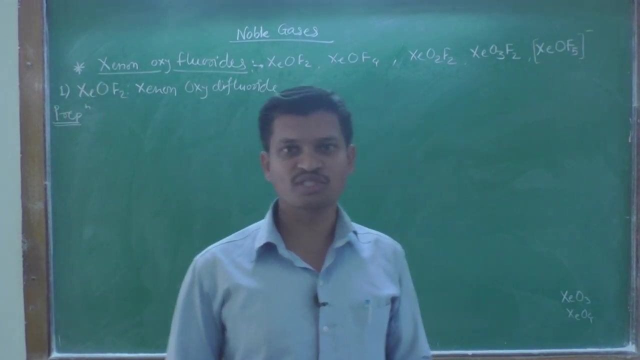 And some ions will be formed, and one of the example is xenon oxy pentafluoride- xenon oxy pentafluoride anion. So we will see, one by one, the preparation methods and the structures of these xenon oxyfluorides. 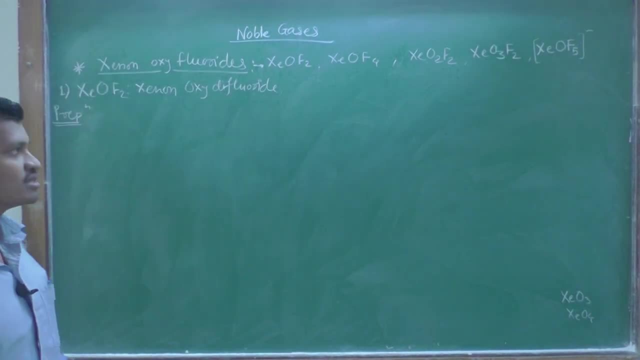 So first one is xenon oxydifluoride. Okay, The formula is XCOF2.. So how will you prepare this? Very simple, Let us start with xenon tetrafluoride. Xenon tetrafluoride. 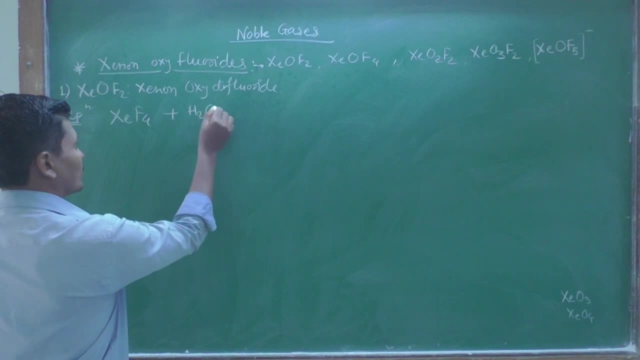 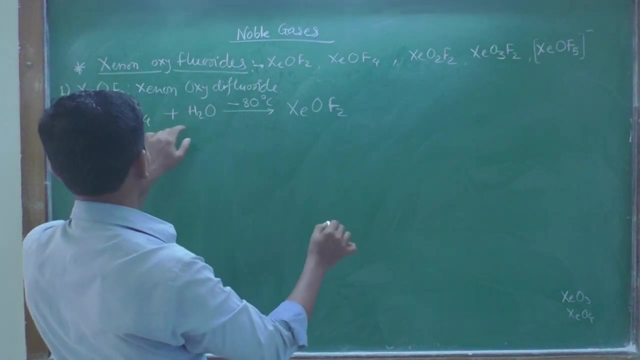 When hydrolysis of this xenon tetrafluoride is done at low temperature, such as minus 80 degree Celsius, then you will get xenon oxydifluoride, Then you will get xenon oxydiachloride XC. as it is. 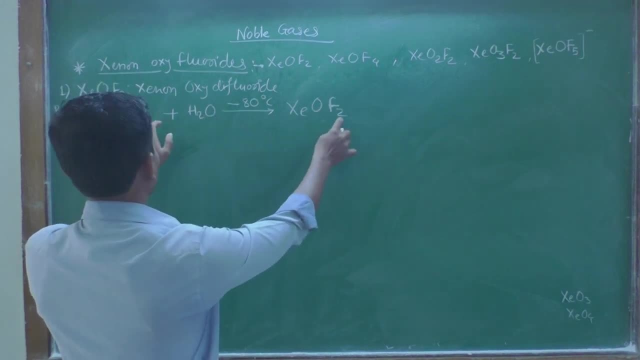 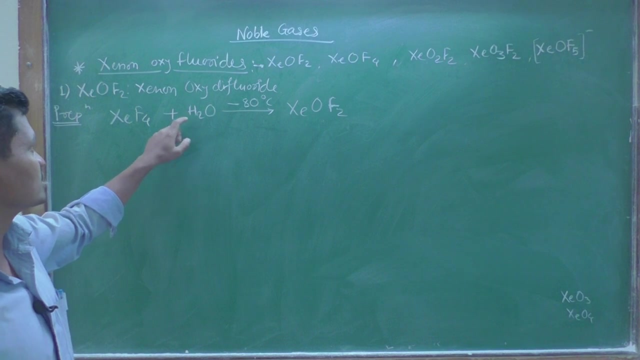 O, as it is F2.. Okay, so in the reactant side there are four fluorine atoms and on the it is also having two hydrogen atoms. So out of four fluorine, Two fluorine comes in the xenon oxydifluoride. 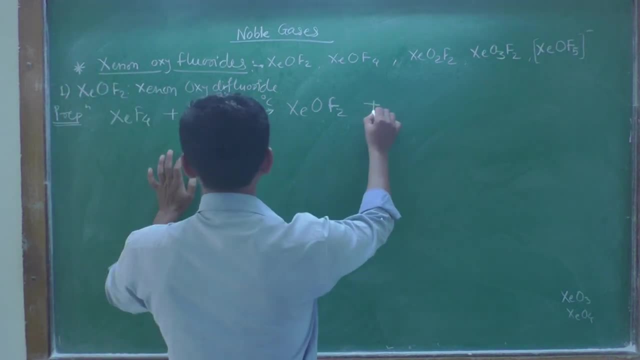 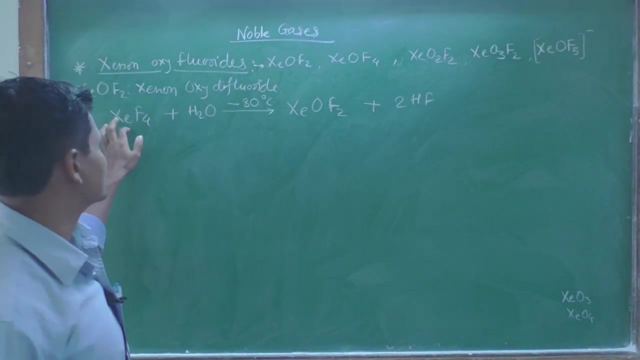 So two fluorine are remaining with two hydrogens, So site product is twice HF. okay, Hydrogen fluoride is the site product. So in this way xenon oxydiachloride can be prepared by using two hydrogen atoms. OK. 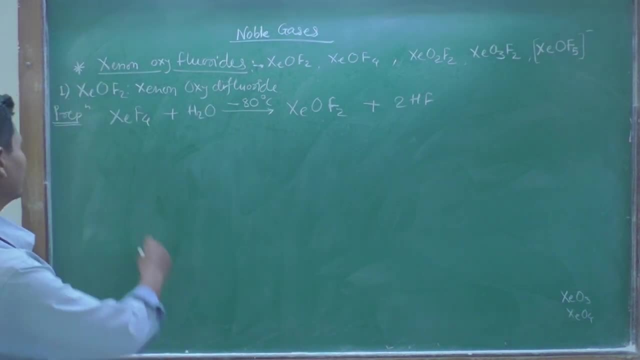 So you can see right, So we can see the hydrogen. Okay, xenon tetrafluoride. okay, now the structure. so the structure of this xenon oxidifluoride can be studied, can be explained on the basis of VSAPR. 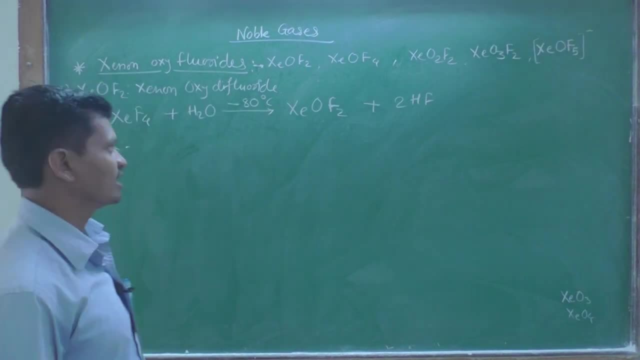 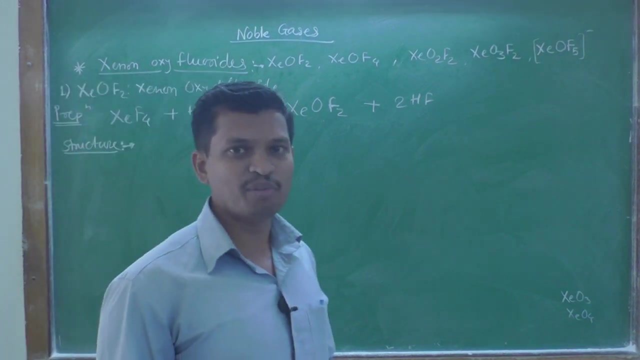 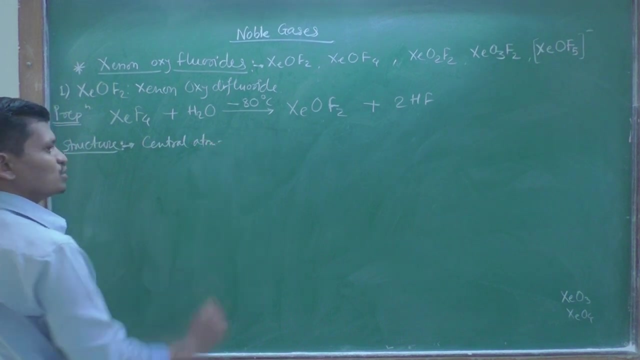 theory: okay, valence, shell electron pair repulsion theory: okay so, and it is also explained on the basis of VBT, that is, valence bond theory. okay, so, the central atom, in this case central atom. so how will you choose? central atom, the least electronegative, thus atom which is having least electronegativity can be. 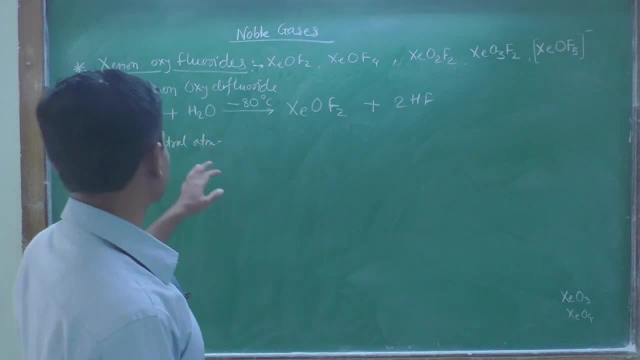 considered as a central atom. okay, so in this case the central atom is general, having least electronegativity, because oxygen and fluorine have more electronegative atoms. okay, now the outermost electronic configuration. outermost electronic configuration of this xenon is 5s2, 5p6 and 5d0. okay, so this is outermost electronic configuration as. 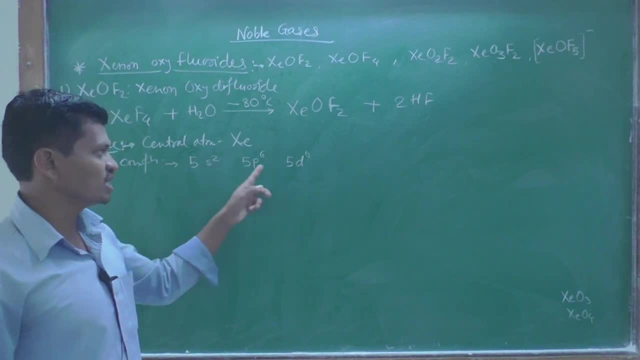 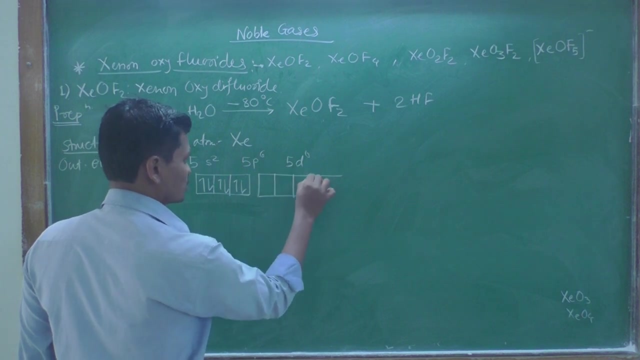 xenon is belonging to fifth period, so its outermost electronic configuration is having fifth shell. okay, so we can dictate this with the help of orbital diagram. so this is 5s2, then p self-shell is having three orbitals. all are fulfilled, okay, and D or, but D substantial is empty. 1, 2, 3, 4 and this is fire D substantial. 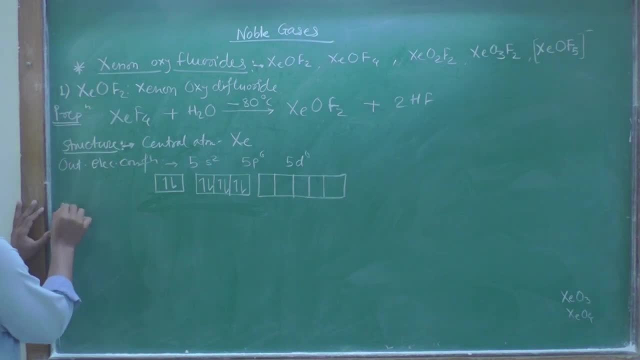 is empty. now this ground state channel is undergoing excitation and hence the excited state electronic configuration will be Like this: So this electron, get this electron and this electron from the P sub cell. they are getting excited to empty D orbital and hence our configuration will become phi S2, phi P4. 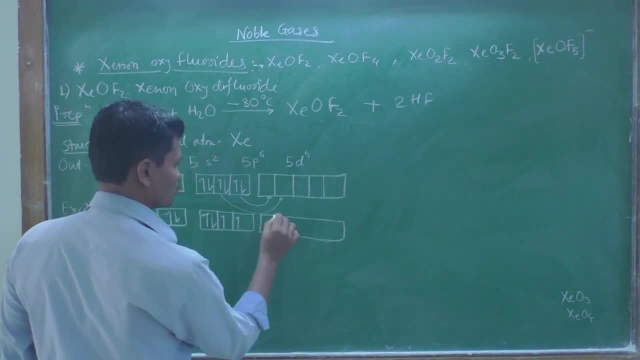 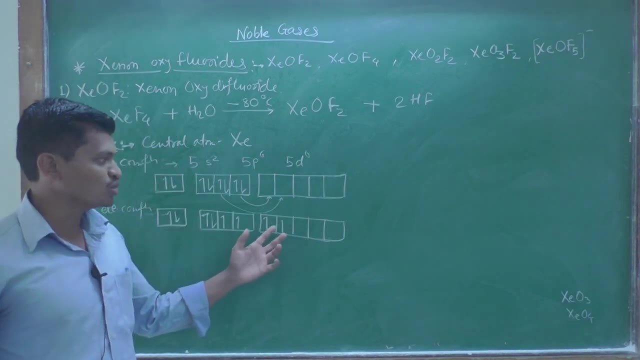 And phi D2, 1, 2, 3, 4 and 5.. Okay, So now we have two electrons in D orbital, So 1 S 3 P and 1 D. 1 S, 3 P and 1 D orbitals get hybridized together, and hence we can write hybridization, hybridization. 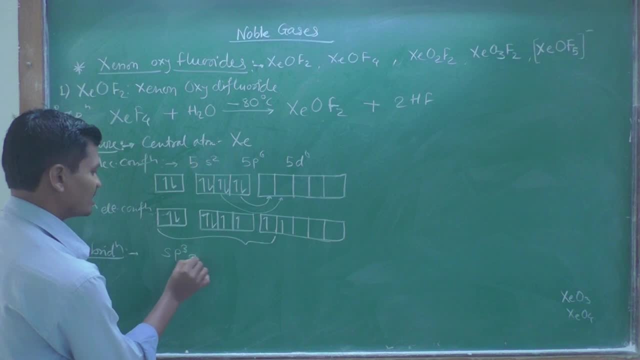 So hybridization is S P 3 D, S 3 P and 1 D S P 3 hybrid orbital hybrid orbitals and they are forming S P 3 hybrid orbitals. So we can 1, 2, 3, 4 and 5.. 1, 2, 3, 4 and this is 5.. So out of these 6 orbitals having electrons, only 5 orbitals get hybridized together. 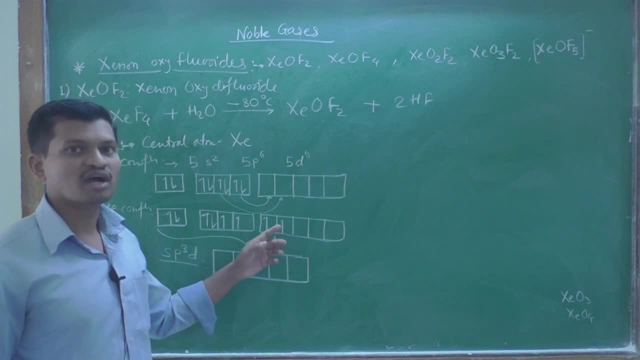 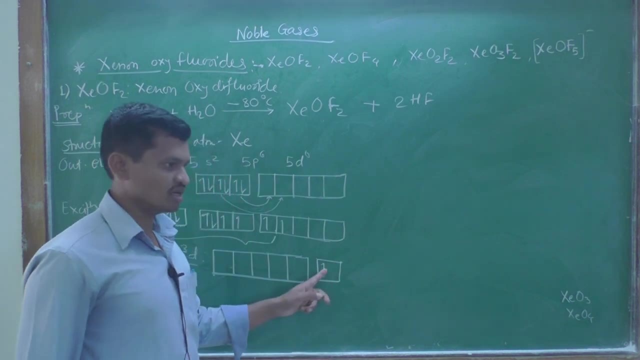 Leaving behind 1 orbital with unhybridized state. So this is the D orbital with unhybridized D. unhybridized D orbital. Okay, So this is S P 3 D hybrid orbitals, 5 out of them. out of them, 1 is having lone pair of electron, 2 of them having lone pair of electron, and 1, 2 and this one is 3rd. Okay. 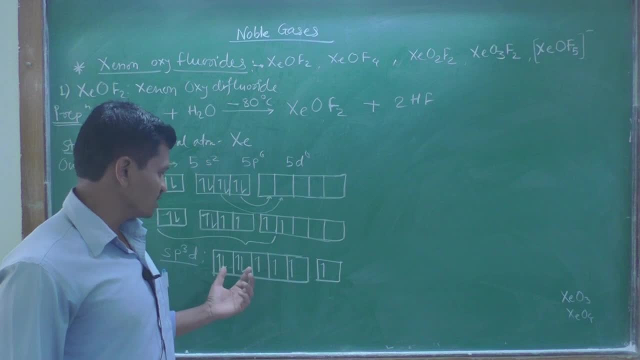 So, out of these S P, 3 D hybrid orbitals, the 2 orbitals are having paired electrons and 3 orbitals are having unpaired electrons, single electrons. Now we have- this is all about xenon. Now we have 2 fluorine and 1 oxygen atoms. Okay So the 2 fluorine atoms- I am showing the cross electrons of fluorine by cross. Okay, So they get shared. the electrons of fluorine are get shared, single electrons are get shared by the 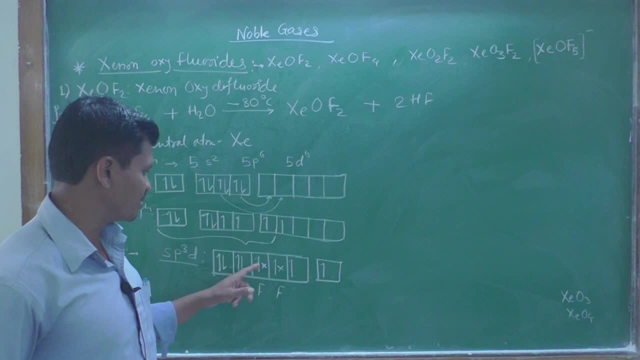 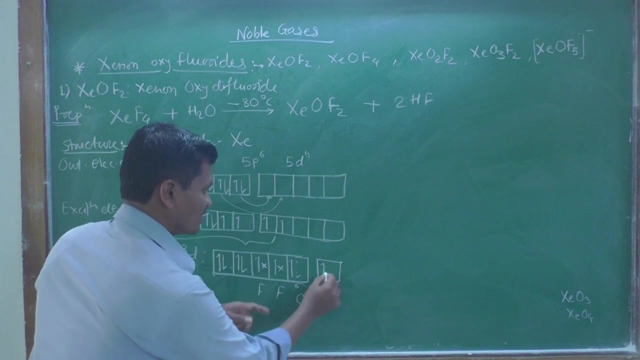 Xenon orbital electron: Okay, S P. 3 hybrid orbital electron: Okay, So 2 fluorine atoms: Okay, As well, as there is a presence of 1 oxygen atom. So this oxygen atom is forming 2 bonds here. 1 is sigma bond with- I am showing it, showing it by dotted arrow: Okay. So this is oxygen atom, It is forming sigma covalent bond and this is unhybridized orbital of xenon, So it is forming a. 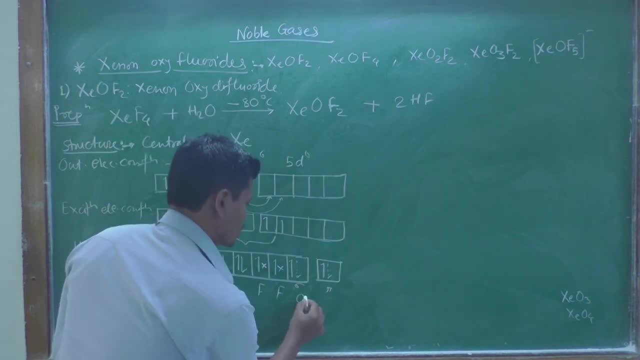 Pi bond. It is forming a pi bond, So both these bonds are formed by the oxygen atom. Okay, One is sigma and another is pi bond. Now, this is S P 3 hybrid orbitals. Now the we will count the number of bond pairs. So now, how many number of bond pairs are there? 1, 2, 3.. So, 3 sigma bonds. are there 3 sigma? 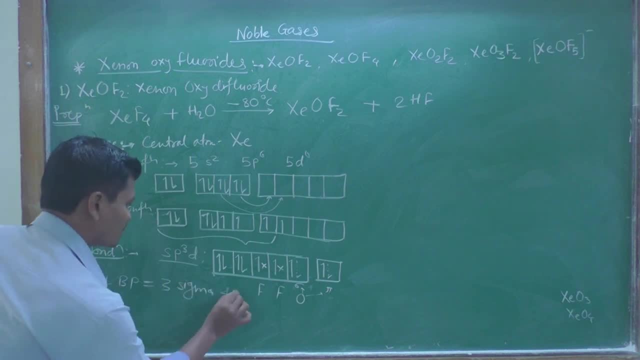 And 1 pi Sigma and 1 pi bond is there Now. number of lone pairs will be 2.. Number of lone pairs will be 2.. Okay, So 2 lone pairs. So while counting the steric number, we are only considering the sigma bonds. So sigma bonds and the 2 lone pairs, The steric number will be 5.. And as steric number is 5., The expected electronic geometry: 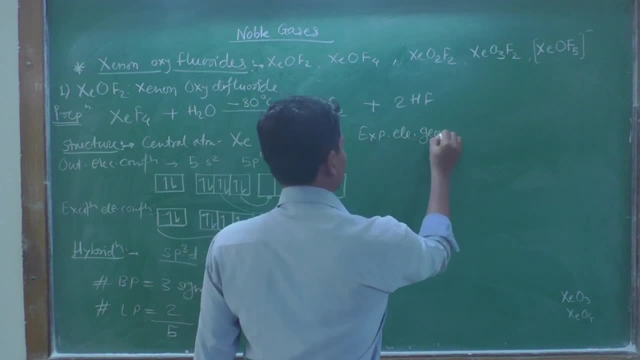 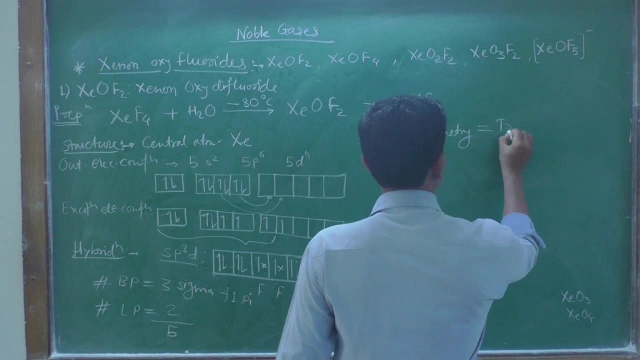 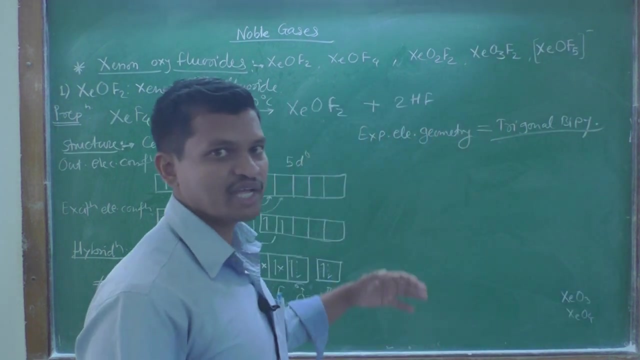 Expected electronic geometry Of the molecule X, C, O, F 2 will be trigonal bipyramidal, Trigonal bipyramidal. This is expected electronic geometry as per the V S, C, P R theory, But while dictating the shape of the molecule or the molecular geometry. 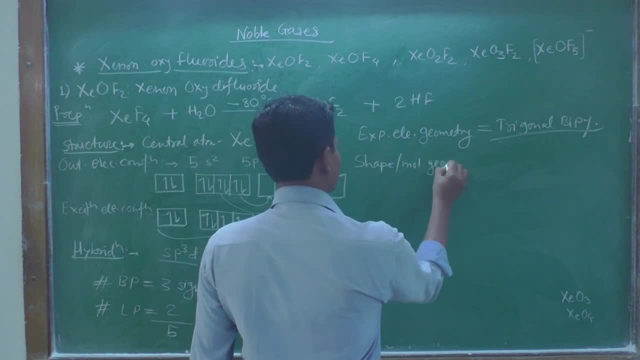 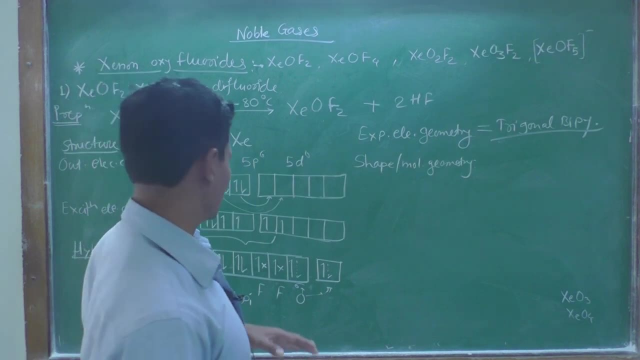 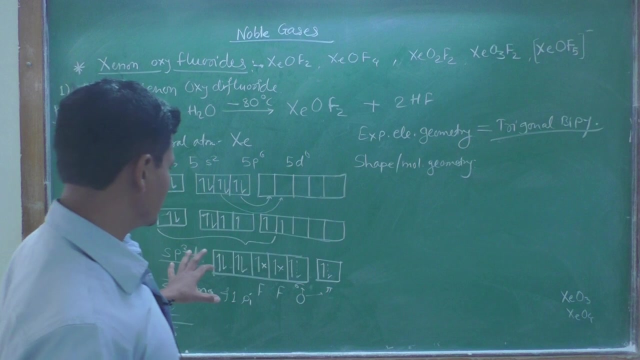 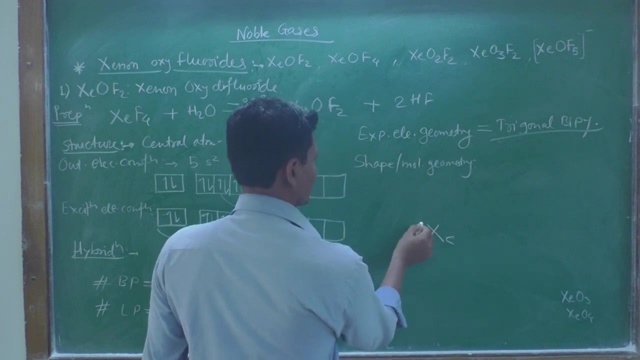 Shape or molecular geometry. We are considering, We are considering only the bond pairs, We are neglecting the lone pairs. Okay, So out of 1, 2,, 3,, 4, 5.. Okay, The arrangement of these electrons, Electron pairs, will be like this. So this is central xenon atom And this is first lone pair, Second lone pair: Okay, 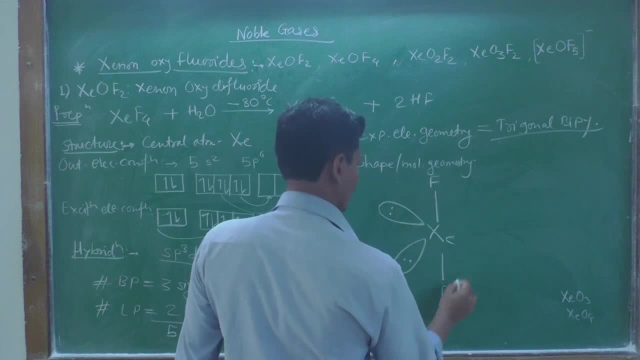 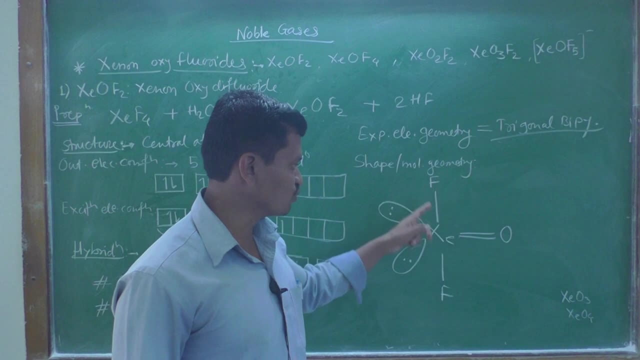 Fluorine, Fluorine, Fluorine, Fluorine, Fluorine, And this is oxygen. Okay, So axial positions are occupied by the two fluorine atoms And the triangular base. triangular base Is occupied by 2 lone pairs. 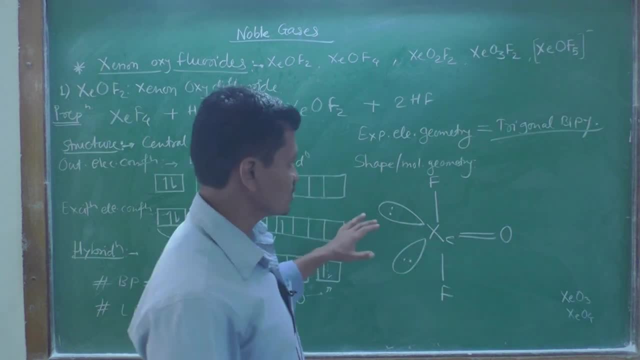 And one corner is occupied by the oxygen atom. Okay, So this is known as trigonal bipyramidal 1,, 2,, 3, 4, 5.. Trigonal bipyramidal, But actual shape of the molecule. 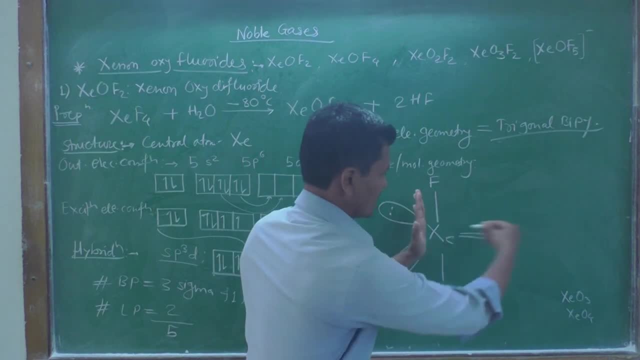 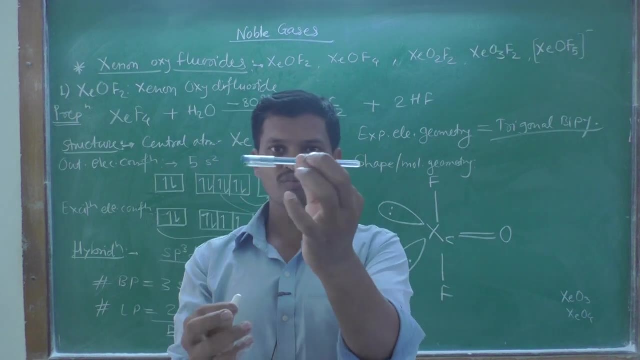 We are neglecting these lone pairs. So it is looking like it is looking like a T shape. So it is looking like a T shape. It is looking like an X, Y, Z, like a t-shape. okay, or we can say that this is the central fluorogenon atom at my fingers. this. 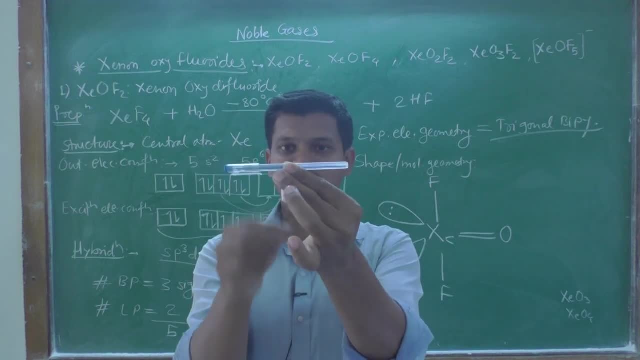 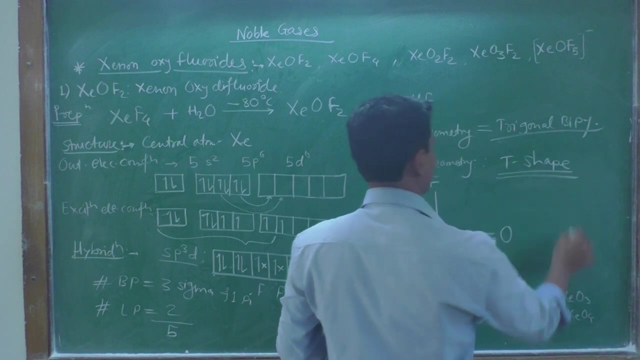 is one fluorine, second fluorine and this is the double bond, oxygen. my chalk is showing the bonding with oxygen and xenon. okay, so this is the shape of the molecule. we call it as a t-shape of the molecule. so shape or geometry of the molecule is t-shape. okay, so this is actual shape of molecule. 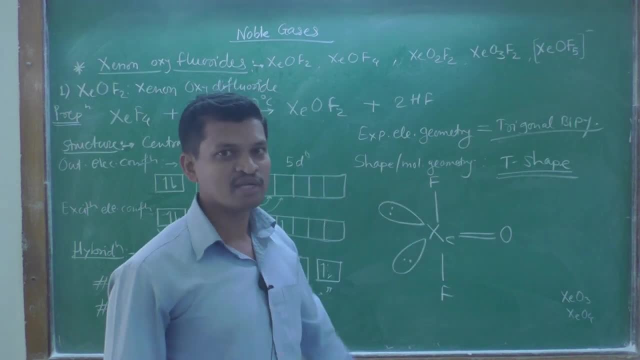 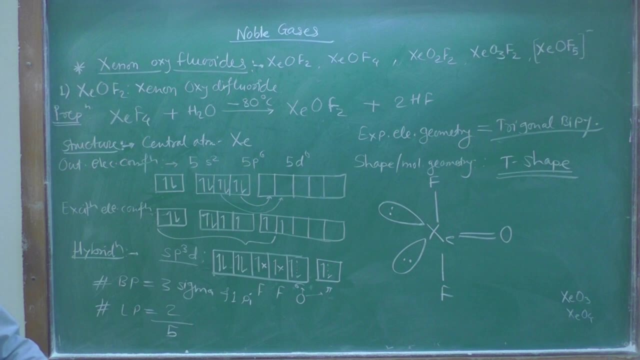 actual geometry of the molecule. we can call it as a molecular geometry. okay, so this is all about the xenon oxy di fluoride. okay. now the second one is called xenon oxy tetra fluoride. xenon oxy tetra fluoride. xeo f4 tetra xenon oxy tetra fluoride. okay, how will you prepare this xenon oxy tetra? fluoride. simply take xenon hexafluoride. do hydrolysis of that xenon hexafluoride okay, and at ordinary temperature it will give xeo f4 plus twice hf, where is easy to remember. only replace tetra fluoride by hexafluoride. 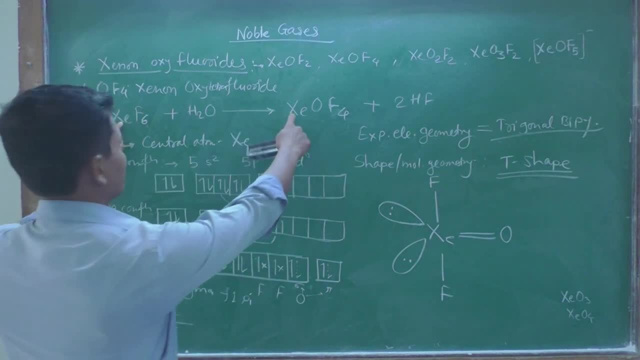 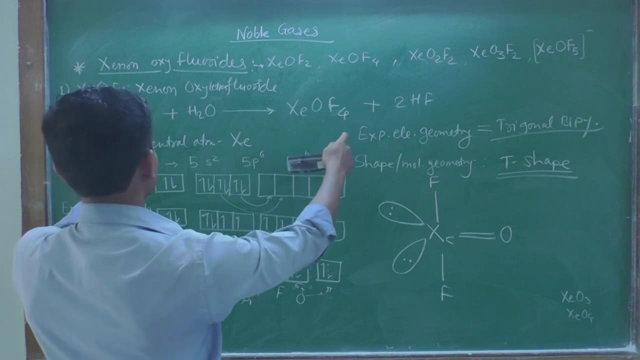 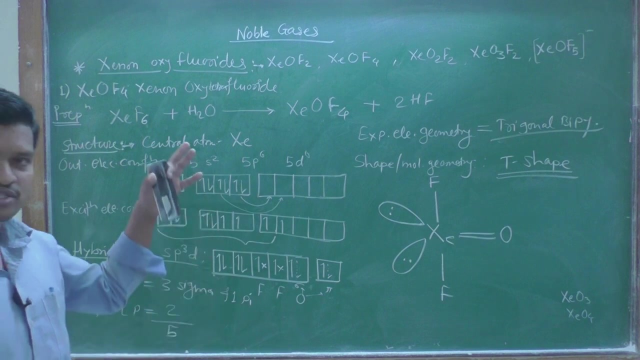 at the starting and you will get xeo. there are six fluorine atoms, out of which four coming in. the product to atoms remains. they combine with two hydrogens forming twice hf. okay, again, the structure will be same and can be explained in the same manner that we have explained for a, for that of xeo f2. 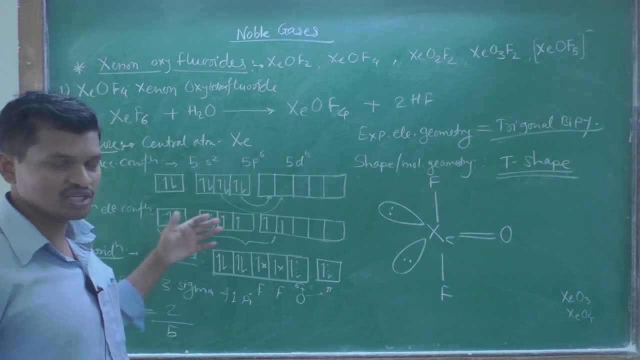 okay, central atom is xenon: outer electronic configuration, then excitation, then hybridization. okay, so what are the changes? that i am only explaining you, okay. so in this case, all the five uh, all the six orbit out of the six orbitals, three or uh out of the six electrons in the 5p. 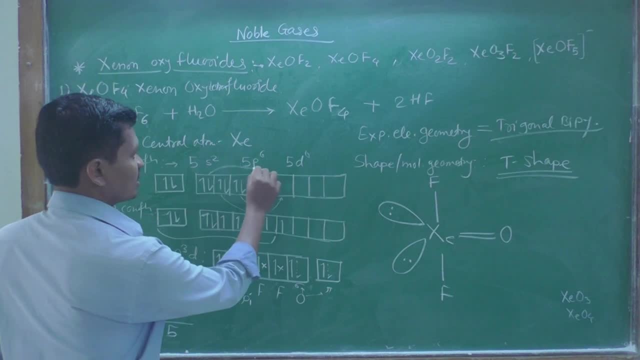 orbital, three electrons are get shifted to the mtd orbital. okay so, this electron shifted here, this electron get excited here and this electron is also get excited to here. okay, so my situation will be: we have to remove this electron and put this in the mtd orbital. okay, so my configuration. 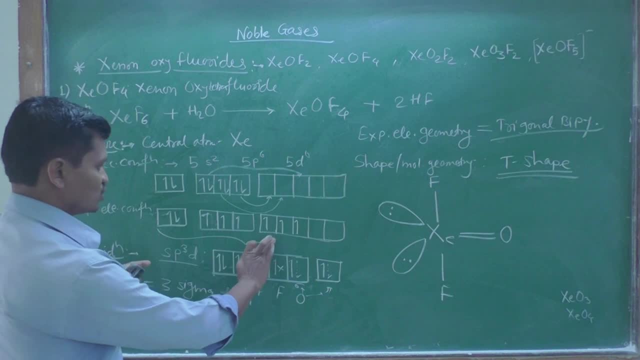 will be. uh okay, so here we have one completely filled s orbital, three completely half filled p orbital and three electrons in the d orbital, so 1s, 3p and 2d. 1s, 3p and 2d orbitals get hybridized together. so my 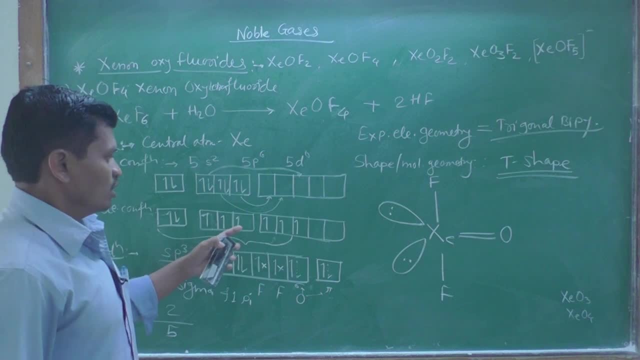 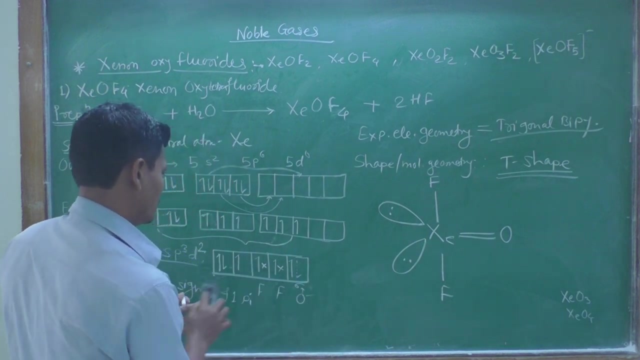 hybridization is sp3 d2, leaving behind one orbital unhybridized state. okay, so this is the hybridization. now, what i am changing to here? only four fluorine atoms. okay, so this is oxygen. this is also fluorine, this is also fluorine, and this is oxygen and this. 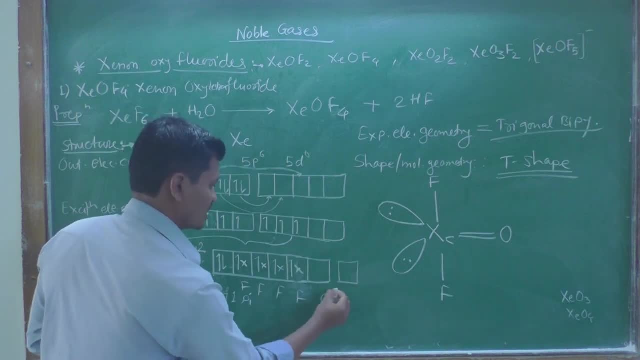 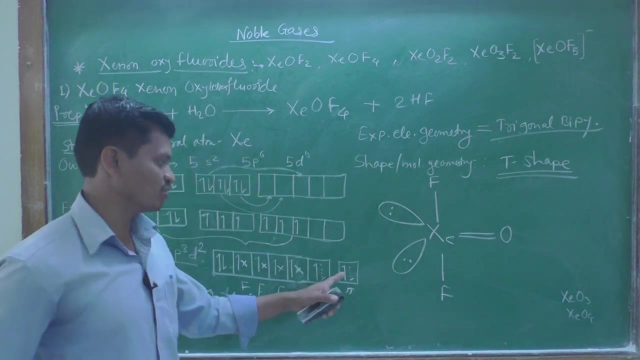 orbital is having. this is in mtd orbital. it is forming a pi bond with oxygen, which is shown by a dotted line. okay, so dotted lines means these are the two electrons that are in the mtd orbital from oxygen atom. okay, one is forming sigma and another is forming pi bond. okay, so pi bond is. 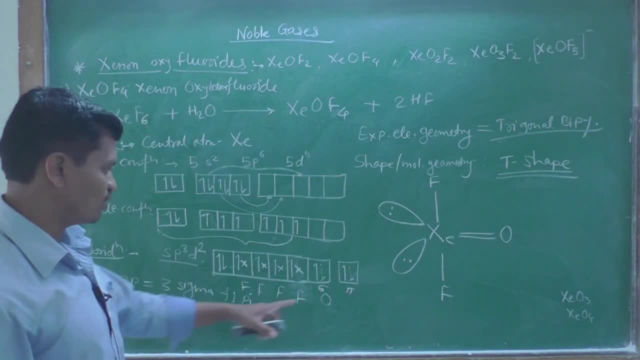 formed by the unhybridized orbital of xenon with oxygen atom. okay, and there are four fluorine atoms: one, two, three, four. the electrons are shown by cross fluorine electrons. okay, so this is the situation, and only one lone pair of electron is there. okay, so number of bond pairs now, uh. 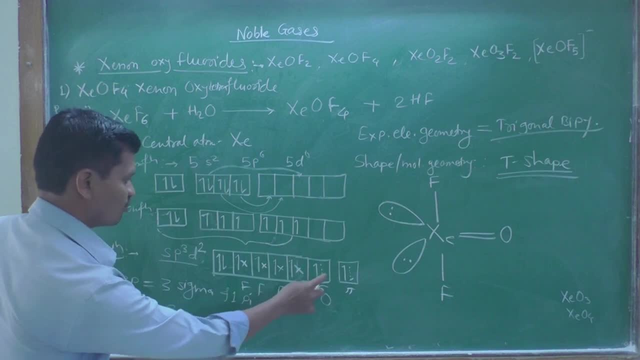 one, two, three, four, five, uh, five sigma, five sigma and one pi five sigma and one, one pi bond, is there? okay, so, and lone pair is only one, lone pair is only one, so five plus six, what is the sum? six, five plus one, six. okay, so the steric. 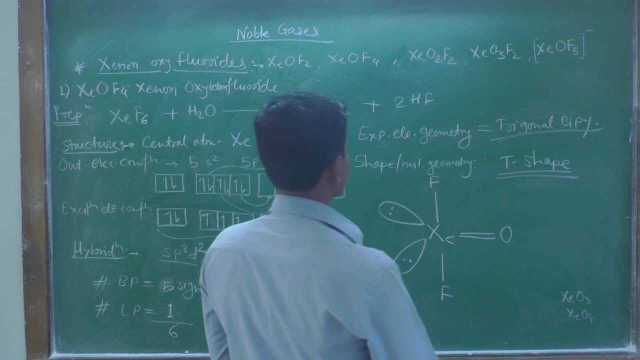 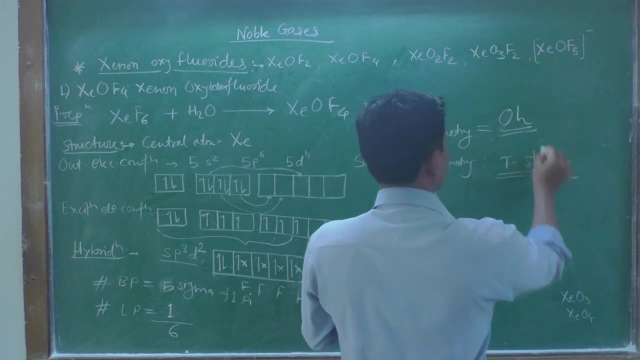 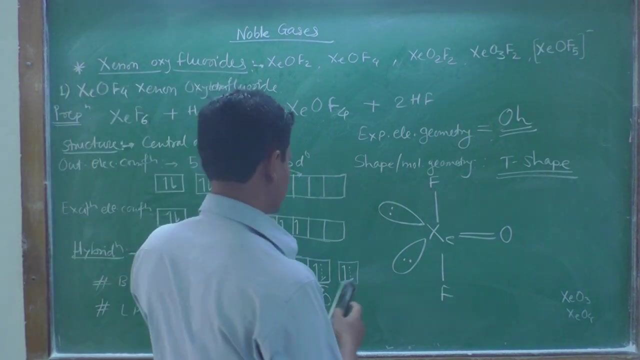 number is six according to vscpr theory. so when steric number is six, the expected geometry is octahedral. expected geometry is octahedral. we are familiar now with this octahedral geometry, so we are trying to uh draw the octahedral geometry of this xco2, xcof4, okay, and 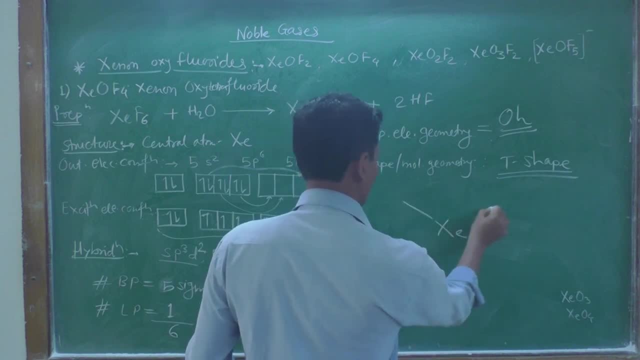 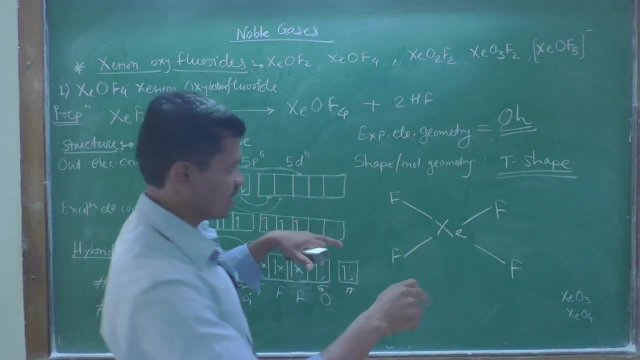 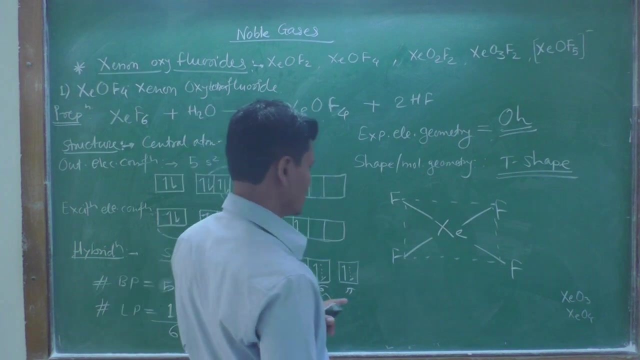 the geometry will be like this: central xenon atom with four fluorine atoms taking a place of four corners of a square planar. four corners of a square planar. okay, so this is a base- what we call square plane, of four fluorine atoms and one oxygen atom is there, so it is taking a axial position. it is taking a axial position. 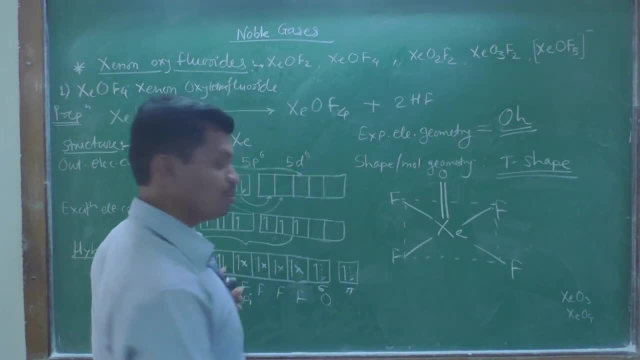 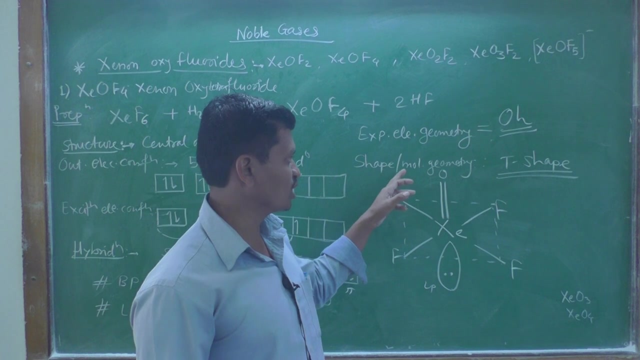 okay, but expected geometry is octahedral. one lone pair is remaining, so put this lone pair at the another axial position. so this is lone pair. okay, so this molecule is looking like a octahedral shape. okay, but actual geometry, or shape of the molecule, molecular geometry, is square, pyramidal. 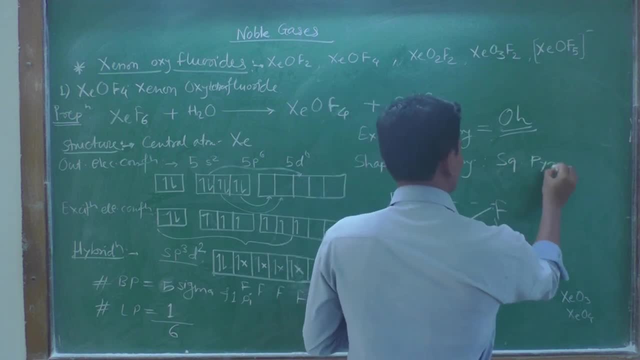 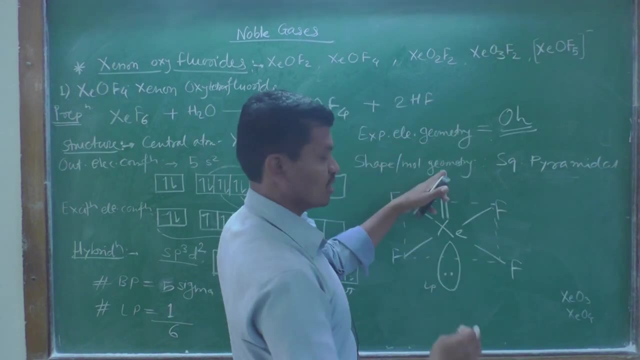 square pyramidal. how will you obtain this square pyramidal? so this is a square and this is only one. bonding is present at the top, so it is a square and it is like a pyramid, square, pyramidal. okay, so neglecting this lone pair, so the geometry will be. 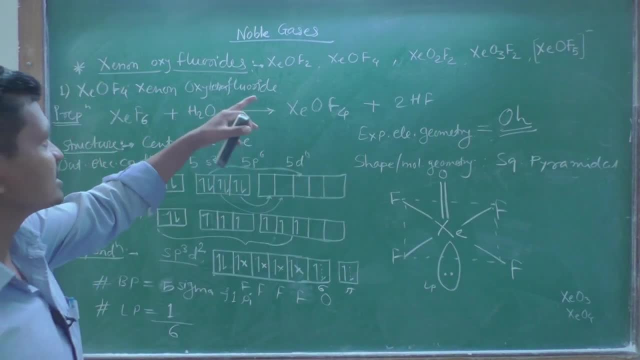 square, pyramidal. okay, so this is all about the xco f4, that is, xenon oxy tetra fluoride. okay, now the last molecule, sorry, next molecule is the xco2 f2. xco2 f2, so xenon dioxide di fluoride, xenon dioxide di fluoride. okay, so the filtration, preparation of this general oxy. 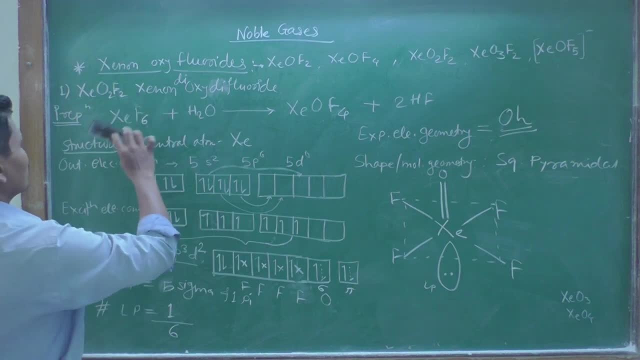 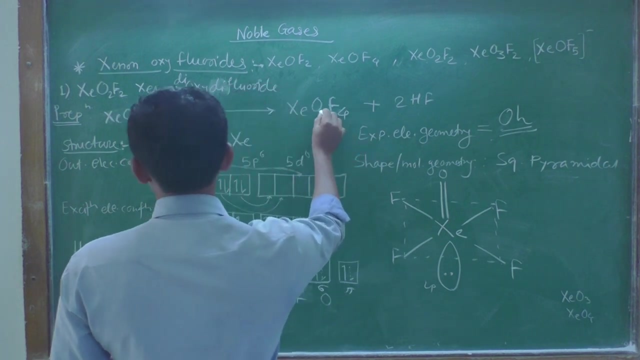 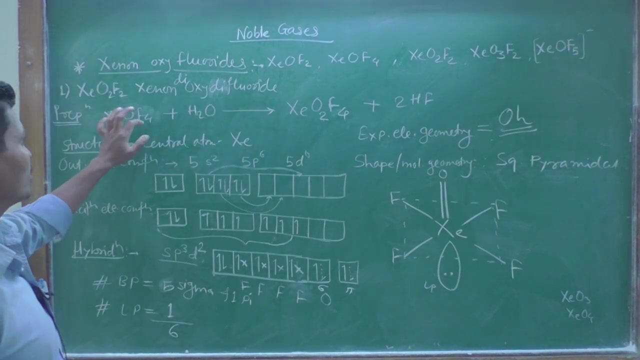 xenon dioxide di fluoride will be from xc f4, xco f4 and xco f4, that is, that is, from this molecule xco f4. react with this water, it is forming xc, o2, f2 plus choice, hf. okay, so from this molecule, we are preparing this molecule xco f4, reacting with water. it is. 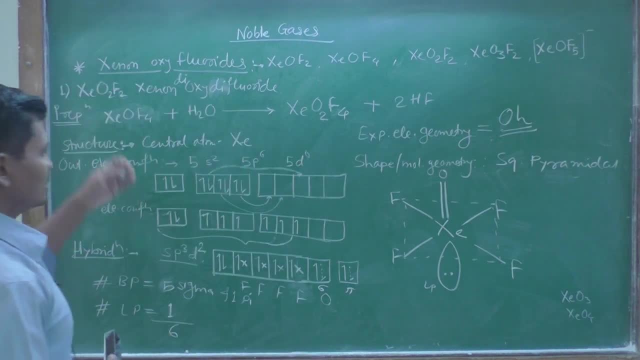 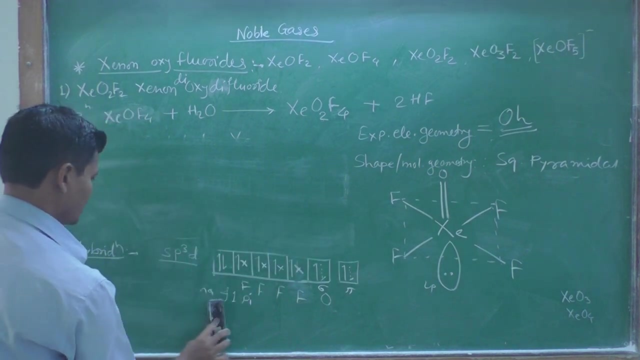 forming xco2 f4. okay, you can try by your own, all these things. okay, i am explaining only here the hybridization and the geometry of the molecule. okay, so in this case the hybridization is again sp3d. hybridization is sp3d- okay, sp3d hybridization- okay. so how many orbitals are? 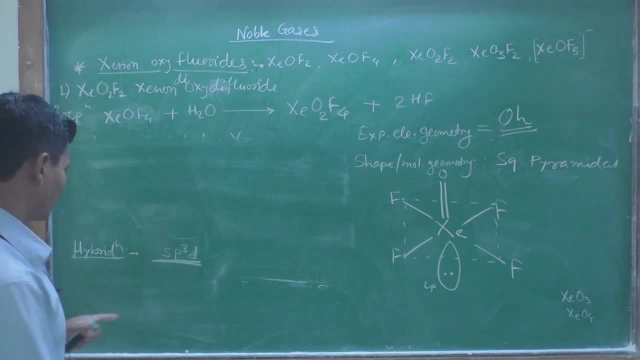 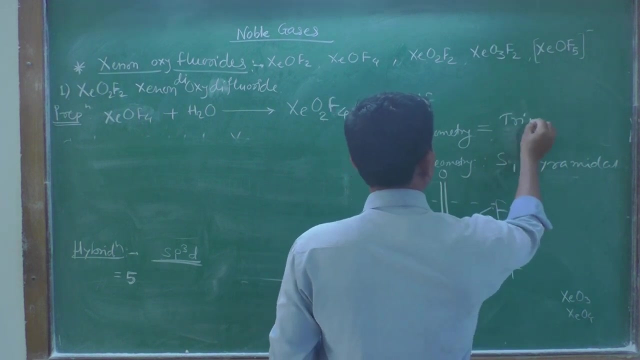 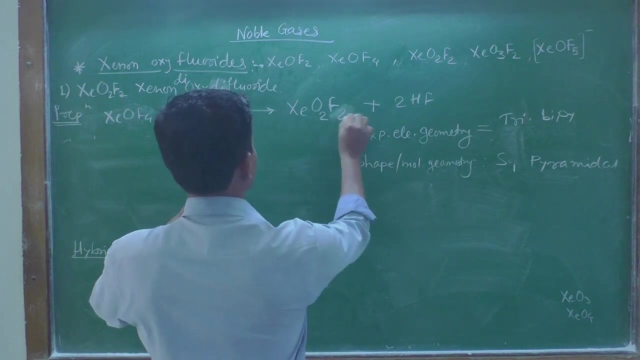 combining one, two, three, four and five. okay, five orbitals are there and now expected geometry of the molecule is trigonal bipyramidal. trigonal bipyramidal as steric number is 5, sp3d. okay, and we will try to draw the structure of this xco2, f2, xco2- sorry, f2 here, xco2, f2, so central xenon with 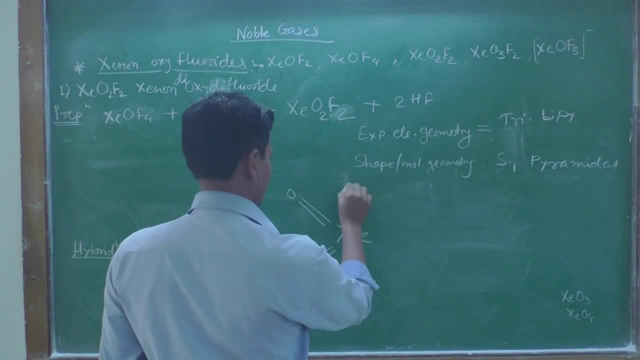 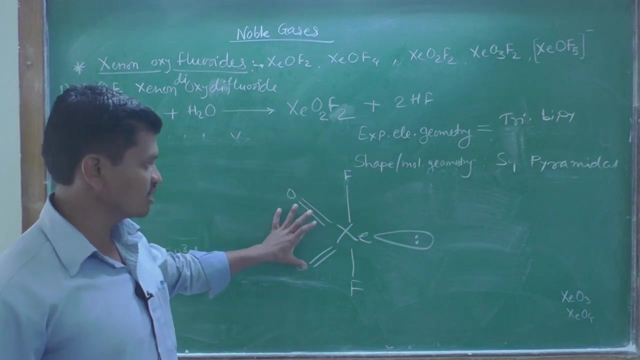 1st siblinguttion and that is the xco2 ketone. what we are getting after this is the xco2 ketone into refractory matrix, and that is why we are using this model over here. we are using this model here, um sorry here: xco2, xco2, xco2. that is our approach. now the third structure. so 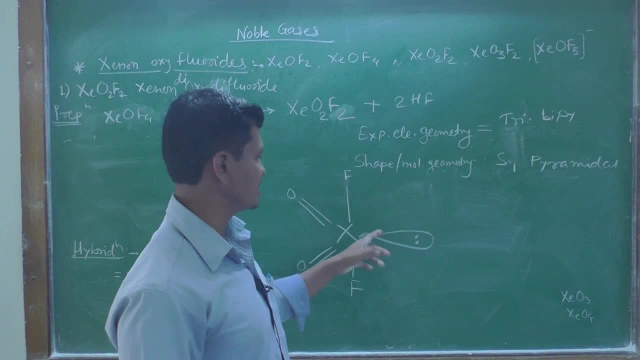 the second structure is Moses H3- situation там- and it is taking the triangular, one of the triangular face or one of the triangular corner. okay, so this is a trigonal bipyramidal looking like a triangular bipyramidal. expected electronic geometry, but neglect this shape. you will looking like this. so it will look like this. 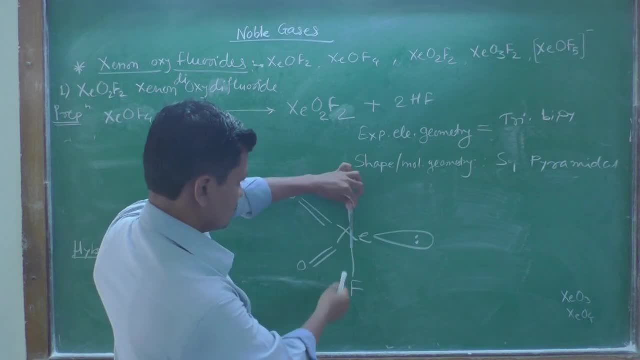 it will look like this: okay, so this is, uh, central xenon atom in my fingers. okay, this is one fluorine, another fluorine and two oxygen atoms. they are like this. so this is the shape of molecule: okay, xenon, fluorine, fluorine and one oxygen, second oxygen. 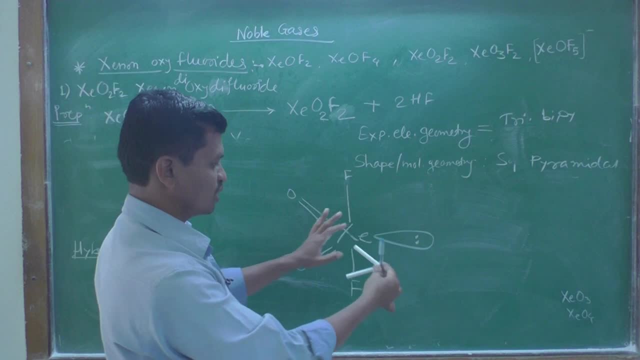 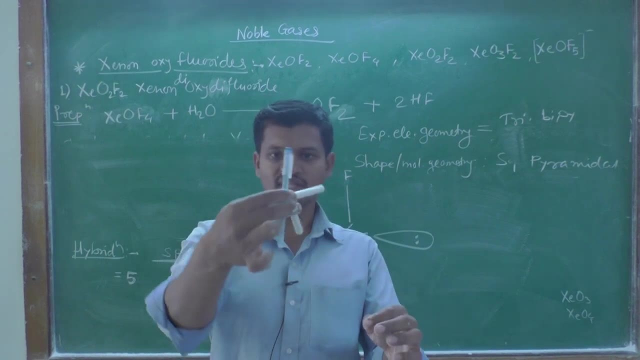 so this is a lone pair. neglect this lone pair for the actual shape of molecule. okay, how will you? looking like this: i am tilting it just like this. okay, so actually it is present. like this: i am tilting it like this: okay, so how it is looking? it is looking like a seesaw. it is looking 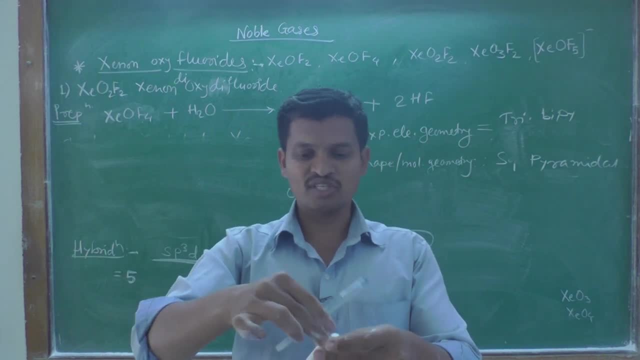 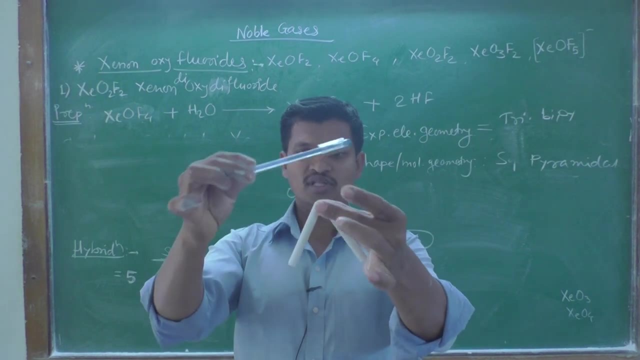 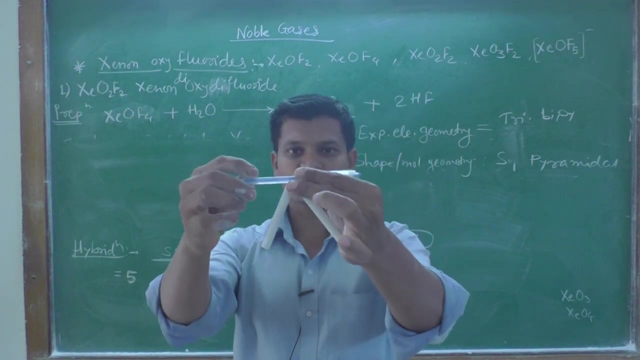 like a seesaw that we are playing in the garden. okay, so seesaw are placed in the garden to play for the little children. okay, and this is the shape of the molecule seesaw. so in my fingers i have taken the xenon atom, fluorine, fluorine with two oxygens, with shown by two chalks. so this is the. 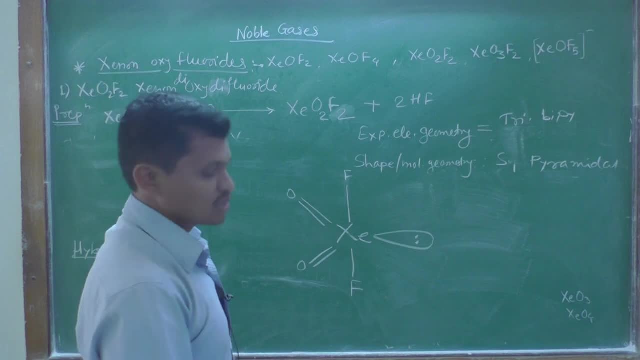 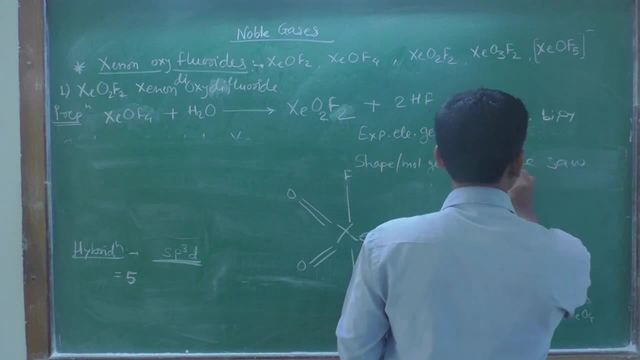 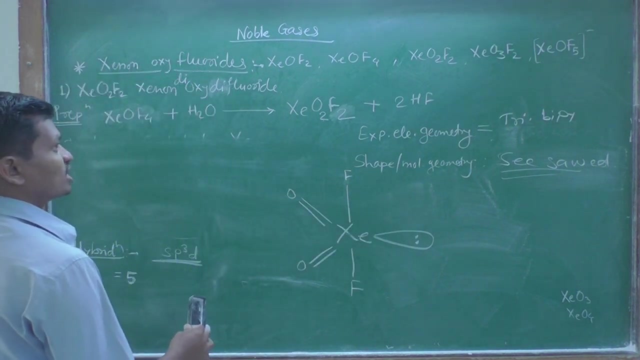 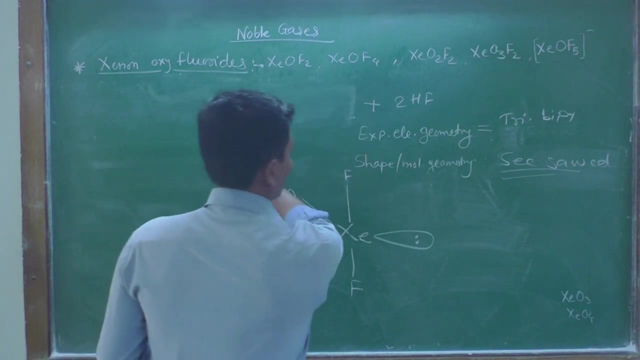 seesaw structure of the molecule. okay, so we can write here: the shape of the molecule is seesaw- okay, seesaw structure- okay. now the next one is xc o3- f2. okay, xc o3 f2. how, what is the structure of this? come to the structure directly: xc o3- f2, so two fluorine. 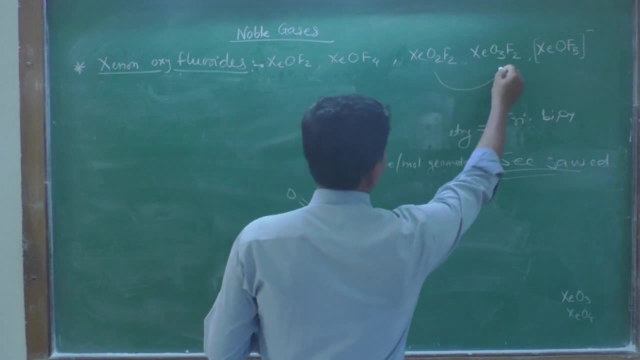 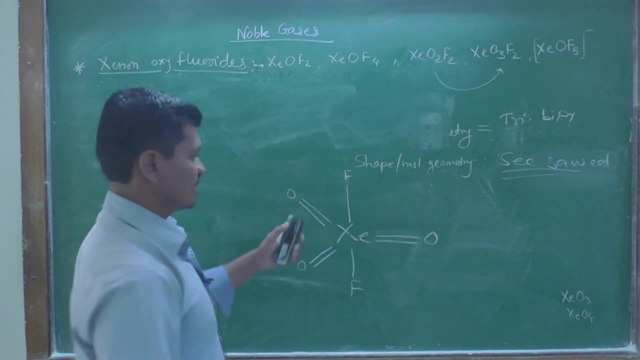 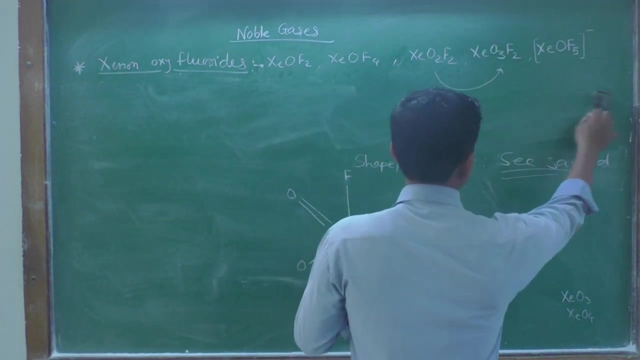 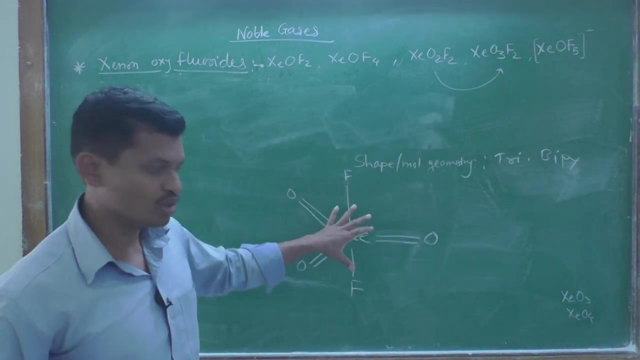 atoms are as it is, so add only one oxygen atom. so replace this lone pair and put a oxygen atom. okay now the expected geometry and the actual geometry, that is, shape of the molecule. both are same, and that is, that is, trigonal bipyramidal, trigonal bipyramidal: both are same. okay now. 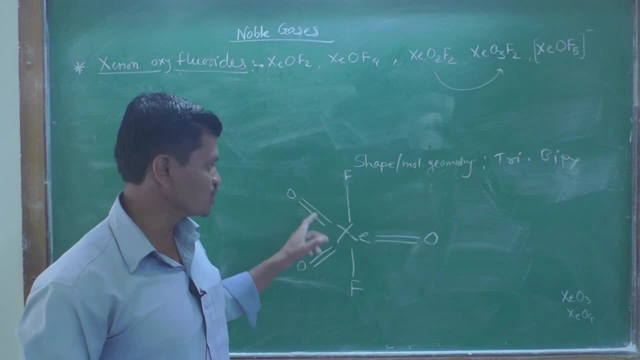 zero lone pairs are present. no lone pair is present in this molecule, so xc o3- f2 molecule is trigonal bipyramidal. next one is xc o- f5, so central xenon atom and one oxygen atom. here you can write that you can divide this in the next one: one, two, three, four. 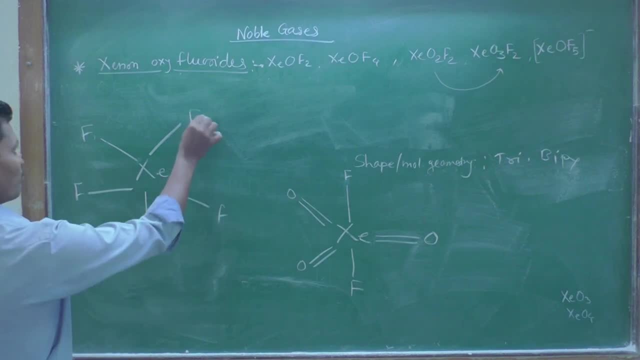 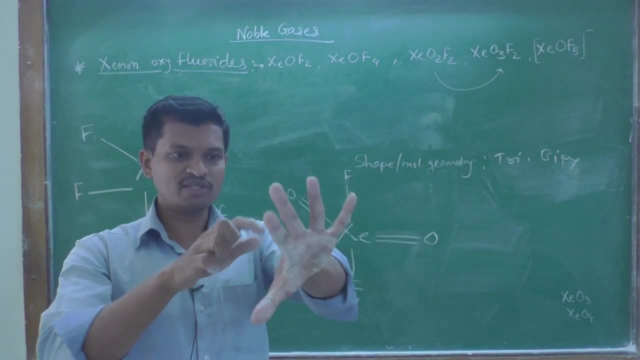 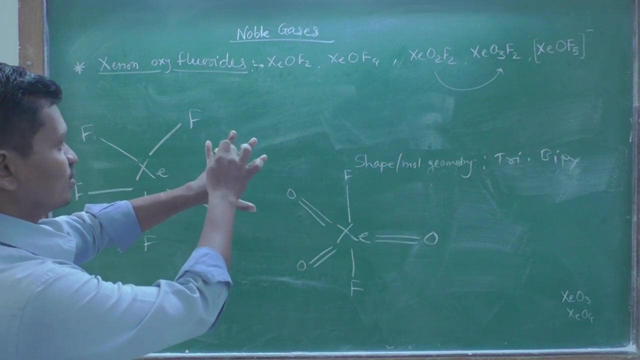 and five, four, five fluid atoms. one, two, three, four and five. five fluorine atoms are present at the regular pentagon- one, two, three, four, five, okay. regular pentagon central. there is a xenon atom. there is a xenon atom at the center place. okay, so this is zenon atom. one, two, three, four, five, okay. 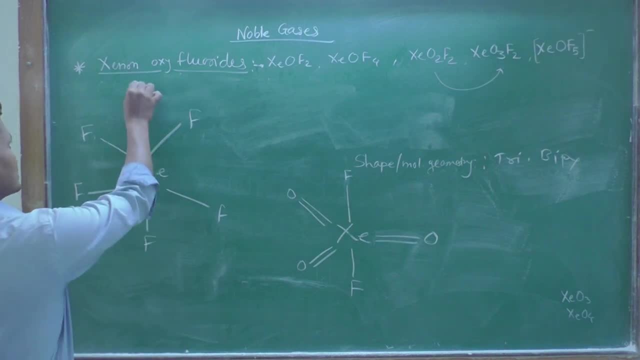 there. so this is taking place, oxygen atom is taking place taking the position of top, okay, and hence as well as there is a presence of one negative charge to this anion, so we can write this: that the structure of the molecule is pentagonal, pyramidal. 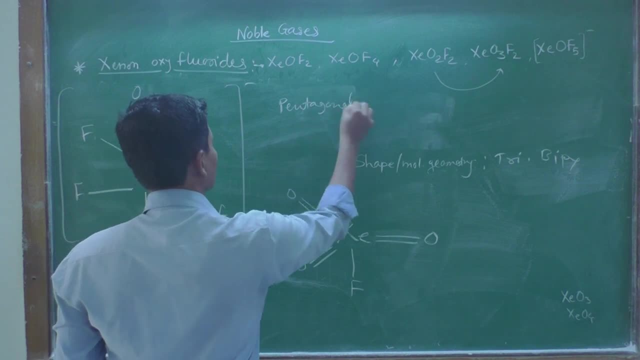 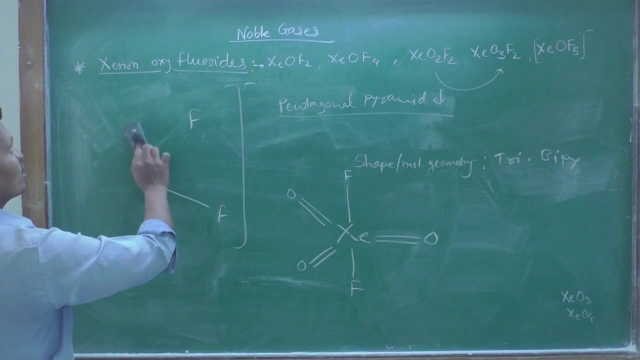 pentagonal pyramidal. this is the shape of molecule: pentagonal pyramidal. okay, so such structures can be asked in your examination for the drawing or identifying. okay, now, these are xenon oxy fluorides. now we have to consider about xenon oxides. xenon oxides. 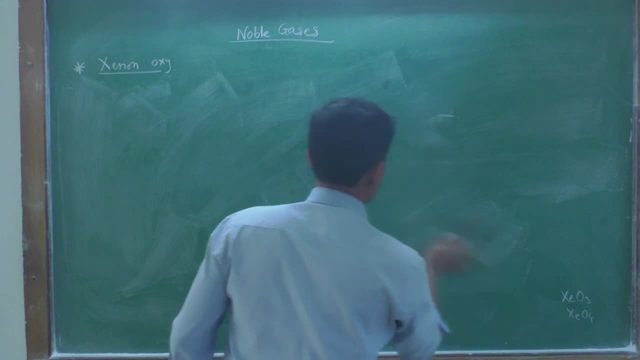 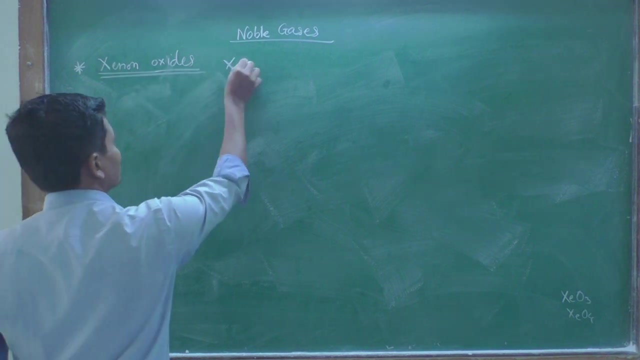 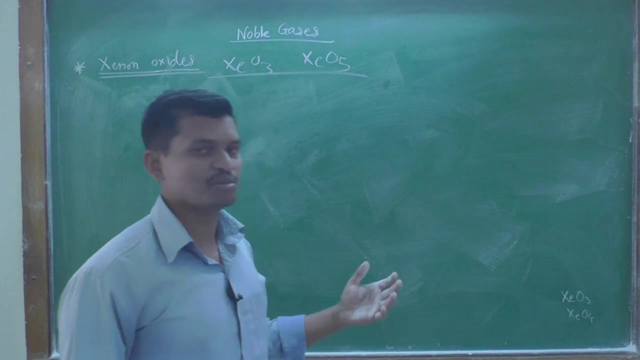 xenon oxides, so XCO 3 and XC o file all the explanation regarding the regarding this structures, how the structures can determine for XCO 3 and XC o. for sorry then, on trioxide and xenon tetroxide, is can be explained on the basis of VACPR theory, as 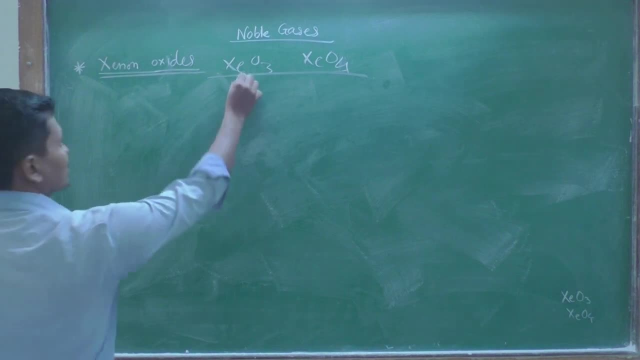 well as VBT theory. okay, So this xenon trioxide, the preparation can be done by using XEF4,. okay, So xenon tetrafluoride, when it is reacting in a proportion of 3 has to 6,. 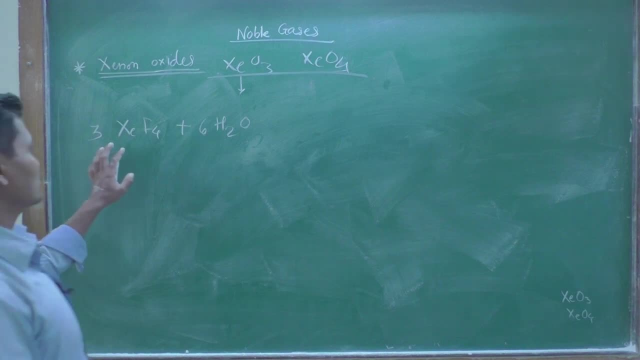 3 has to 6, okay, There is a formation of 2 xenon plus XEO3, okay, So 3 xenon atoms are there. out of this, one is forming 2 xenon atoms and another xenon atom is combining with oxygen to form XEO3. 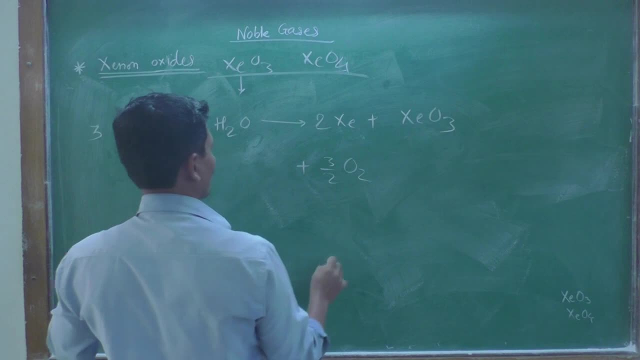 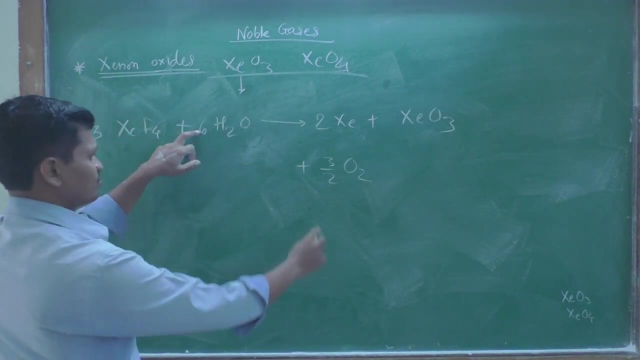 plus formation of 3 by 2 O2, okay, 2 to get cancelled, 3 oxygen remains. So 6 oxygen are there, 3 are combining with xenon forming trioxide and they are forming 3 by 2 O2.. This is a balanced. 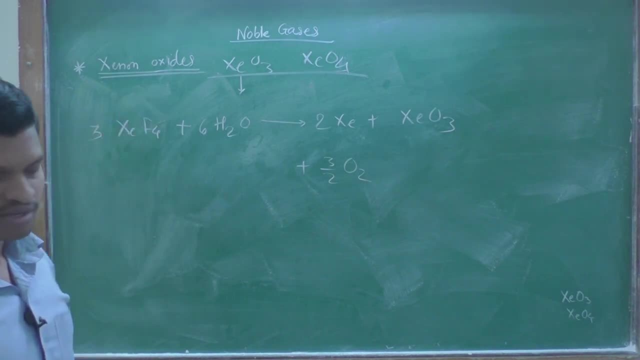 chemical reaction for the formation of xenon trioxide. okay, Now structure. This structure of the xenon trioxide is very important. So this is the structure of the xenon trioxide. So this is the structure of the xenon trioxide. So this is the structure of the xenon trioxide. 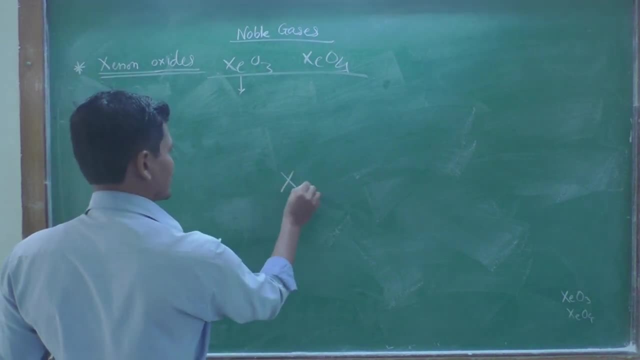 Very easy. Central atom is xenon. It is forming 3 bonds. It is forming 3 bonds with 3 oxygen atoms having one lone pair of electron and that lone pair of electron taking a position of apex. okay, So the hybridization is SP3.. Hybridization is SP3 for central. xenon atom and hence expected geometry. expected geometry or electronic geometry is tetrahedral but neglecting this lone pair, the actual shape of the molecule or molecular geometry is just like ammonia central nitrogen with 3 hydrogens and the lone pair at the apex. it is pyramidal. 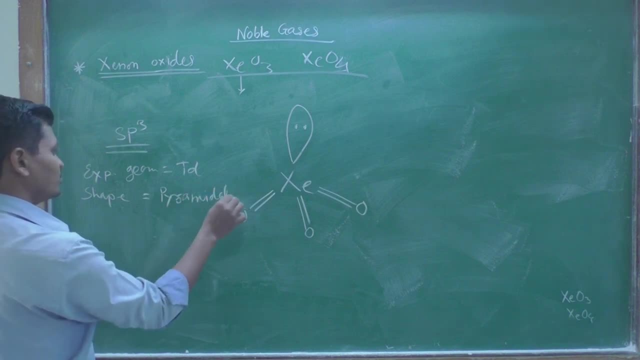 It is pyramidal. okay, So this is the structure of xenon trioxide. You can try to solve this xenon trioxide structure explanation by your own. okay, Just I have explained for the remaining previous examples. okay, So this is xenon trioxide. Now what is the change? 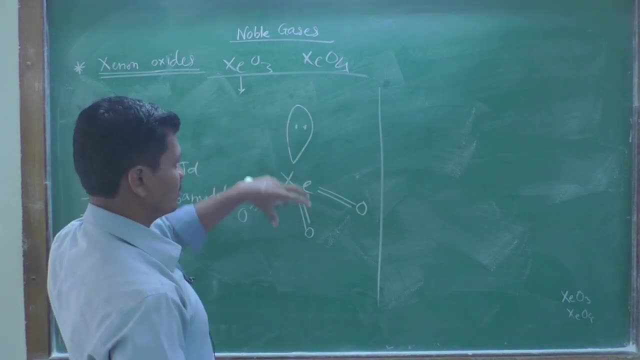 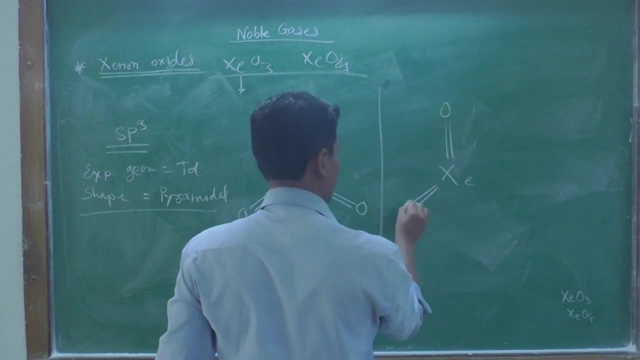 only for tetraoxide. Replace this lone pair at the top and by a fourth oxygen, So you will get xenon tetraoxide. One, two, three and this is four. okay, So this is an actual geometry and expected electronic geometry. both are same, okay, and that is tetrahedral. 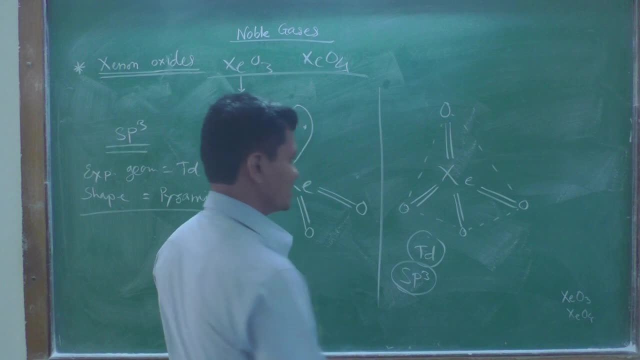 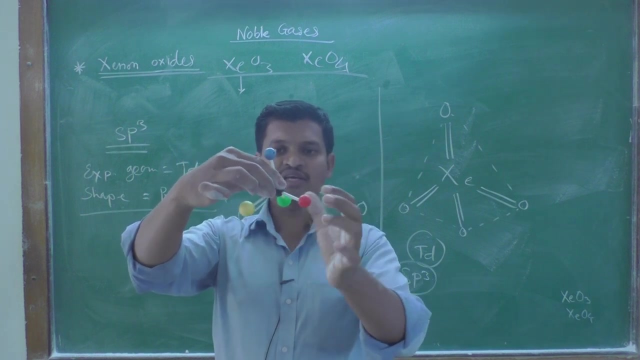 That is tetrahedral. Central xenon atom is undergoing SP3 hybridization, okay, and the shape of that molecule is like this. So this is central xenon atom- black ball in my hand, okay. So this is central xenon atom one, two and three. These are three oxygen atoms. 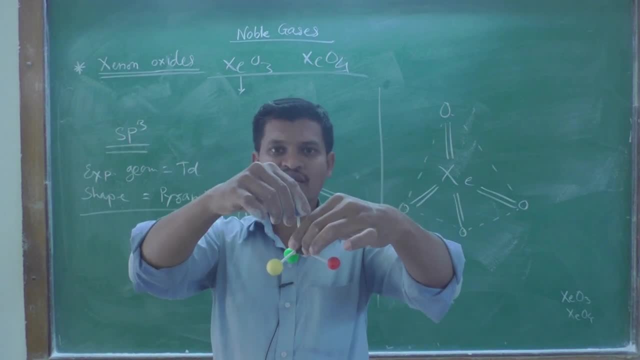 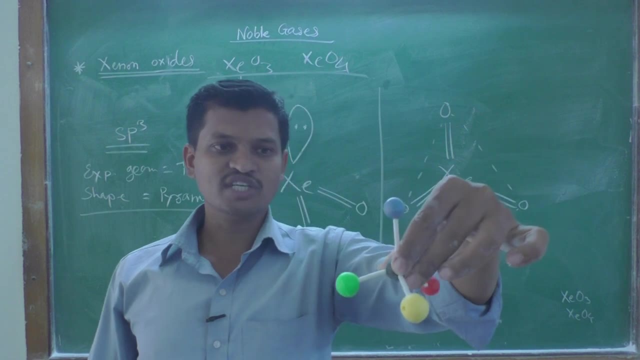 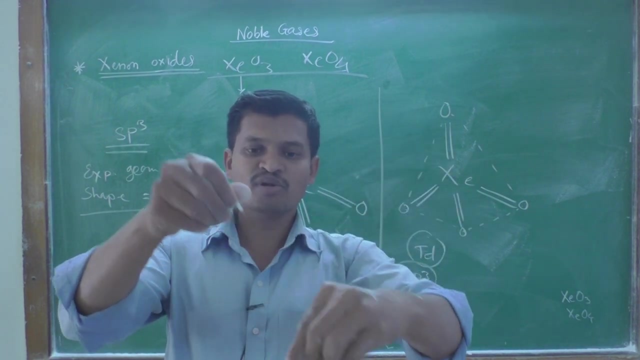 okay, And the fourth one is at the top. So this is a structure of a regular tetrahedron in three dimensions. okay, You can easily judge yourself. that is, how is the structure of this xenon trioxide? It is tetrahedral, and when we replace this top oxygen atom, it is xenon. 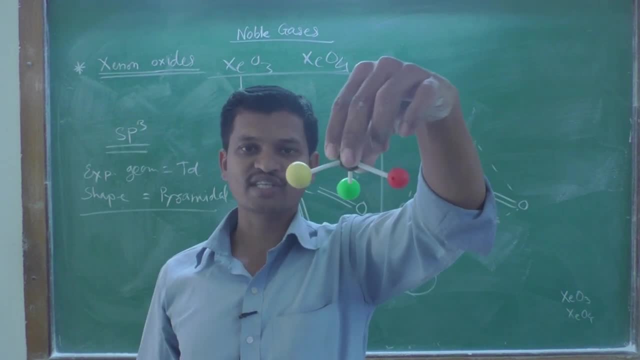 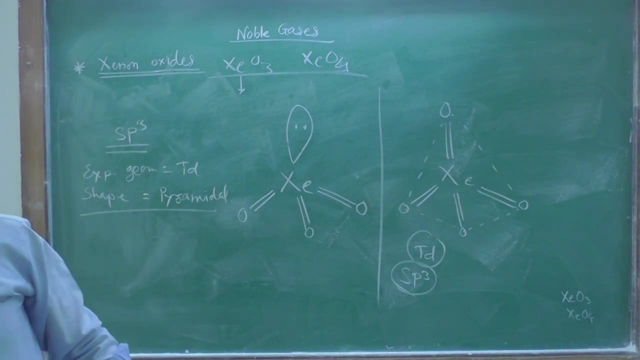 trioxide, XCO3.. It is looking like a pyramidal shape. It is looking like a pyramidal shape. okay, So both structures are very easy to understand. This is the total discussion of xenon oxyfluorides and xenon oxides. okay, So very easy to understand.